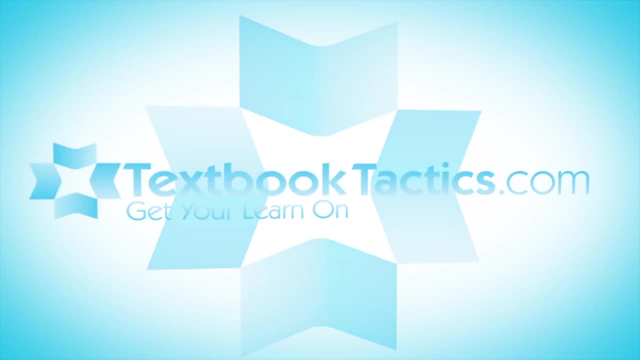 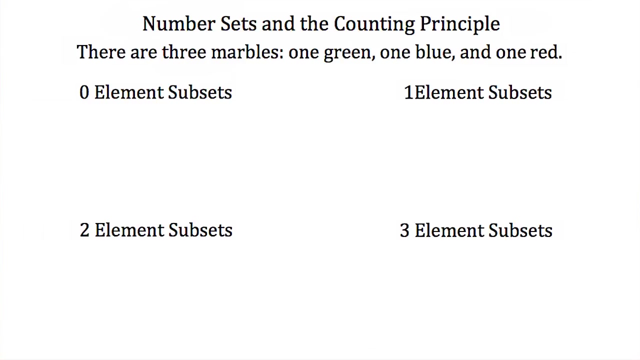 This is a tutorial on number sets and the counting principle. The first thing that we're going to talk about in this tutorial are number sets, and to illustrate a number set, we're going to use a set of three marbles. We have one green marble, one blue marble and one red marble. Now there's lots. 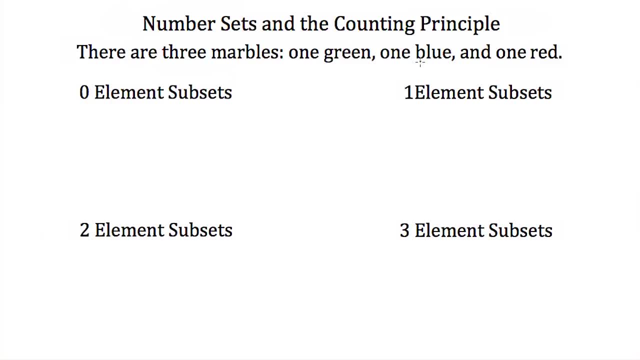 of different subsets that we can get from these three different choice of marbles. These subsets all have zero, one, two or three elements in them, and an element is just a selection, so it would be a marble. If I wanted a zero element subset, well, I would be choosing. 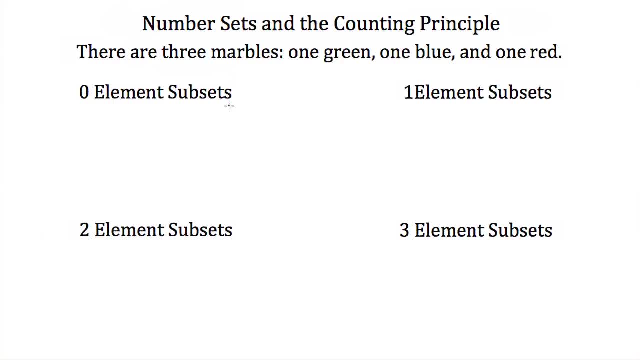 zero marbles out of the three, and there's only one way to do that: I don't choose any marbles. If I wanted a one element subset, that would mean I would choose one marble out of the three possible, and there are three different subsets for choosing one marble. I might choose the green. 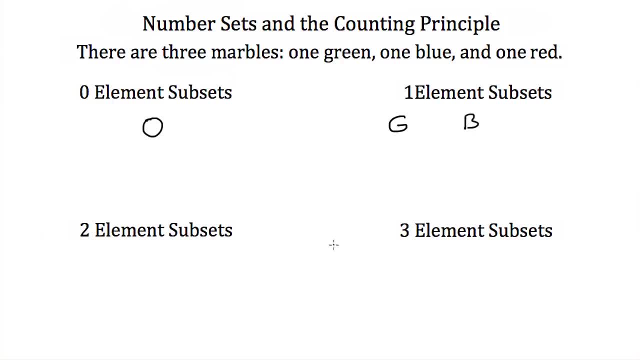 marble, or I might choose the blue marble, or I might choose the red one. So there are three different, one element subsets from these three different marbles, Just like there's only one way to choose zero marbles. Now if I wanted to choose two marbles or 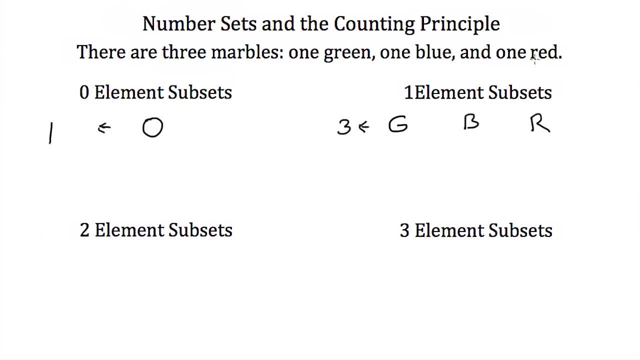 two elements out of the three possible. well, I might choose a green one and then a blue one, or I might choose a green one and a red one, or I might choose a blue one and a red one. Those are the only three ways. I can choose two out of the three marbles. So there are three different marbles. 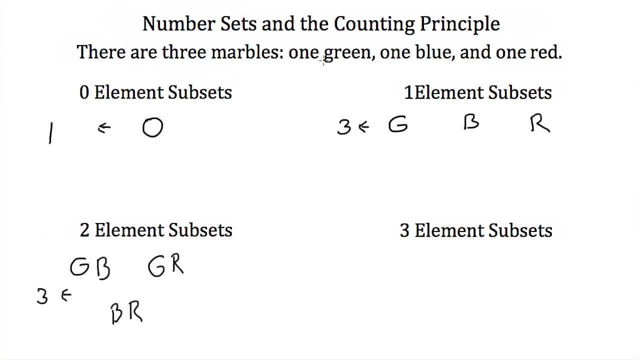 ways to create a two element subset from this set of three marbles. Now, if I want a three element subset, that means I'm going to choose every one of the marbles. I would have a green, a blue and then a red one. So there is only one way to choose a three element subset out of three different elements. 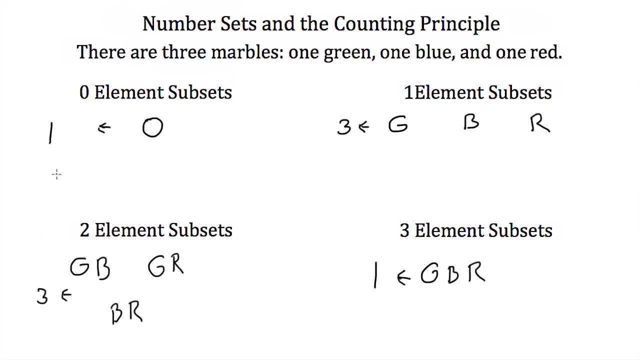 If we add up all of this, one plus three is four. three plus one is four. four and four would give us eight. So there are eight different element subsets for the choice of three marbles. If you have a set, say it's set A, and set A has n elements in it, then set A has two to the n possible subsets. 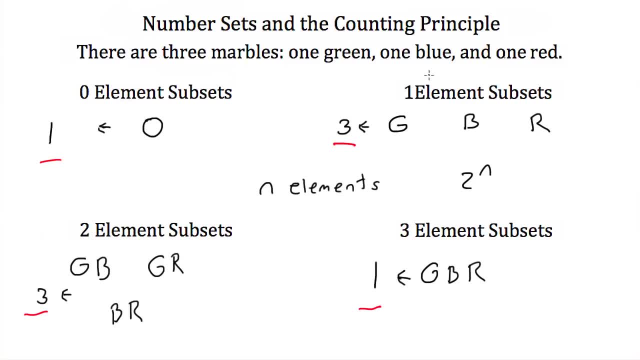 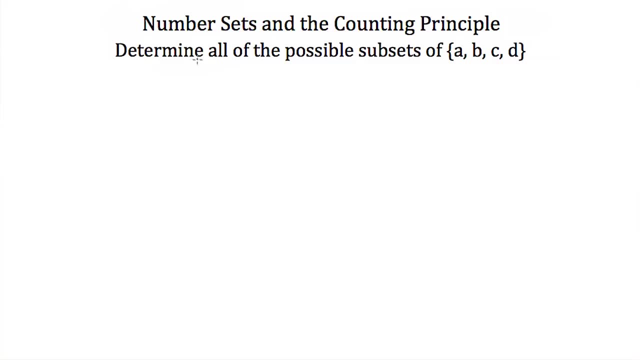 So the fact that we had three different elements in our set of three marbles, we ended up with two to the third power subsets of our three elements, which was equal to eight. So here we're asked to determine all of the possible subsets of this number set that's just listed as A, B, C and D. Well, there are four elements to this set. 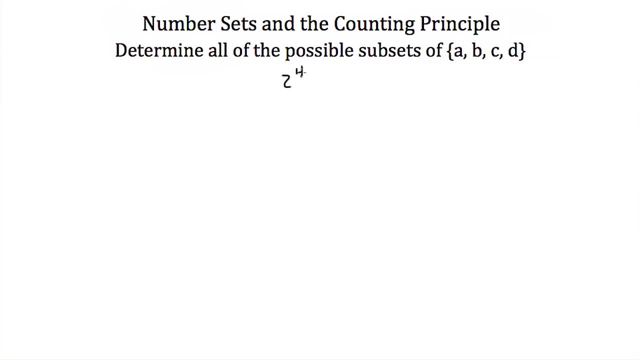 which means we should get two to the fourth power amount of subsets. Two to the fourth power is 16, so we should get 16 different possible subsets of A, B, C and D. First we'll have some zero element subsets and there's only one way to do that. don't choose any of the possible. 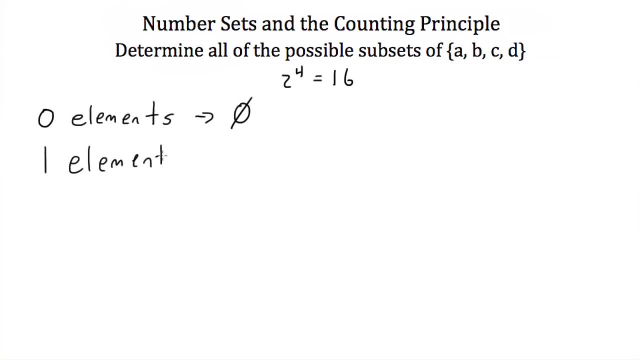 then we might have a one element subset. and how many different ways can we choose one item out of the four possible? well, we might choose A, we might choose B, we might choose C or we might choose D. so there are four different ways to do that. we might have some two element subsets, then we would choose A and B, or maybe A and C, or maybe A and D. 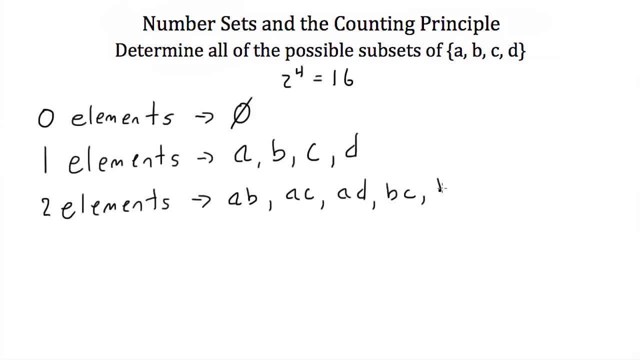 we also might choose B and C or B and D, or we might choose C and D. so there are six different possible two element subsets. now three element subsets. we might choose A, B and C. we might choose A, C and D. we might choose A, B and D. 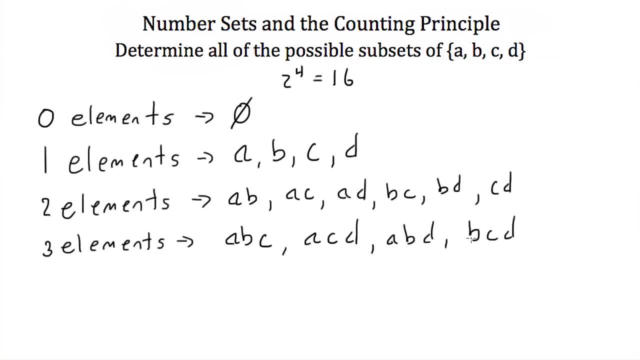 or we might choose B, C and D. so there are four possible three element subsets from this set of A, B, C and D. we have four elements, so there's one more to do a four element subset. well, there's only one way to do that. we just choose every one: A, B, C and D. now let's check our work. there's only one way to choose. 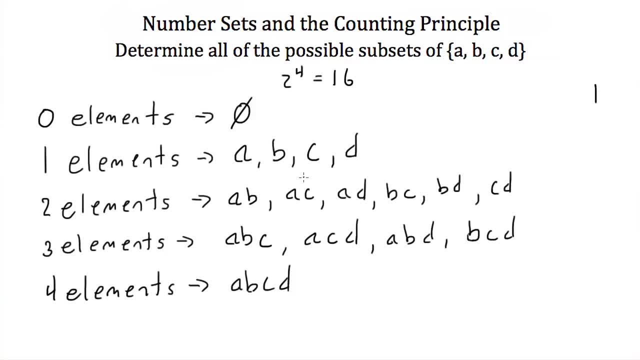 zero elements. you just don't choose any. there's four ways to choose one element. there are six different ways to choose two elements, four different ways to choose three elements and one different way to choose all four. add this all up and it comes to 16.. so we did find all of our possible subsets and they're all listed right here. 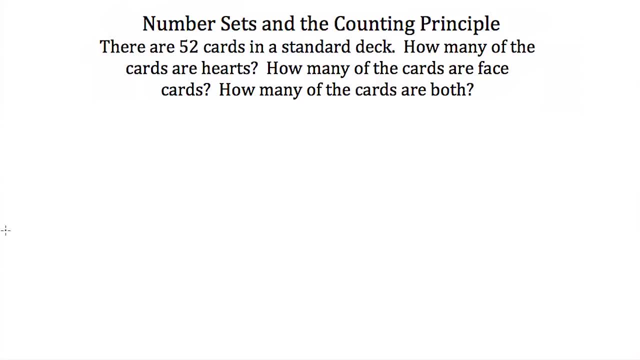 now there are many different ways to illustrate number sets here. we're told that there are 52 cards in a standard deck and we want to know how many of these cards are hearts, how many of these cards are face cards and how many of the cards are both a heart and a face card. 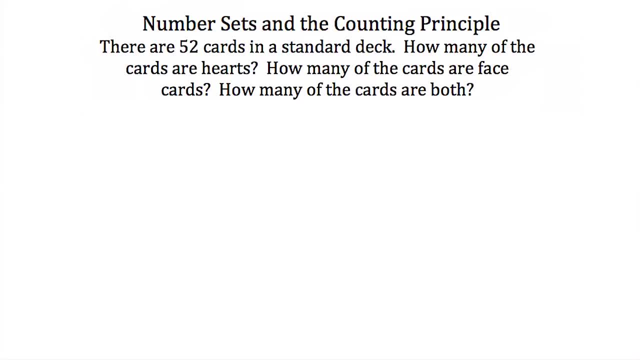 well, a popular way to illustrate a number set is to use a Venn diagram. this is a Venn diagram. this giàmo la dots in it represent each possible card that we might choose out of the deck. Inside this circle there are 13 red or purple dots. These 13 dots represent the 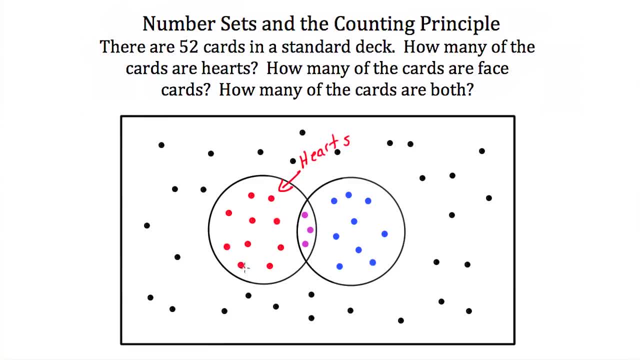 amount of hearts that are in the standard deck. The blue dots represent the amount of face cards that are in the standard deck. These purple dots: they represent the cards that are both hearts and face cards. And then all these black dots are just cards that are neither a heart or a face card. Now there are 13. 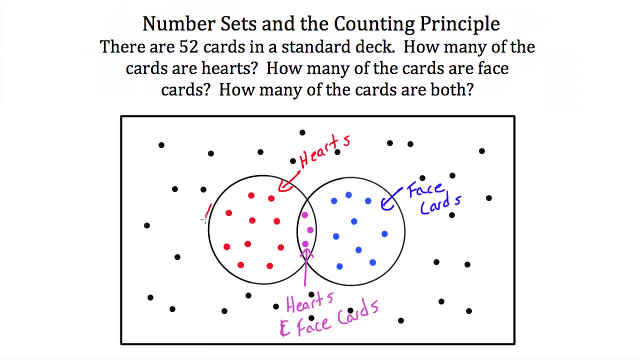 hearts and every point inside this circle here is a heart. There are 12 face cards and every point inside this circle is a face card. Now you'll notice that these three points in the center are actually in both circles. That's why those are the cards that are hearts and face cards, because they're in the heart. 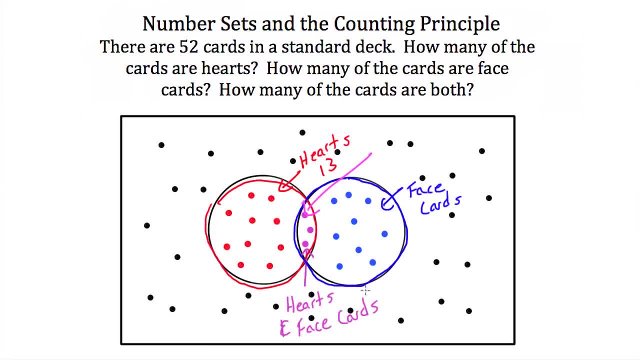 circle and they're in the face card circle. So this is how we use a Venn diagram to illustrate how many of the cards are face cards, or how many of the cards that are hearts and how many of the cards are both. We just create these. 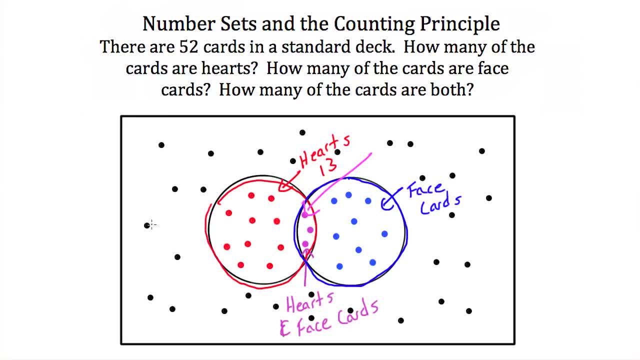 circles, to group the individual possible numbers or sets together. Another way to think of this is to think of a circle as a circle and a circle as a circle. So this is a 52 different numbered set. The hearts are a subset, the face cards are a. 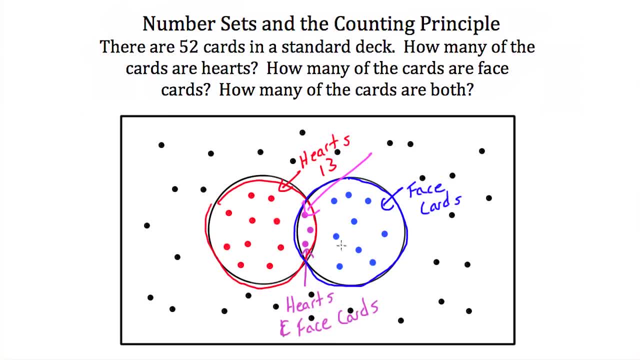 different subset and the combined hearts and face cards are a different subset. Now we're asked how many of the cards are hearts? Well, we can count the dots, or, if you just know, there are 13 hearts. How many of the cards are face cards? 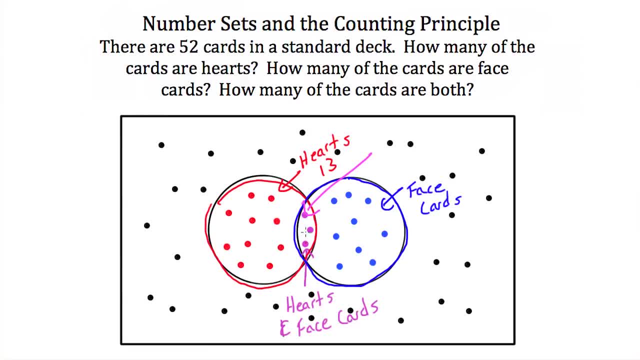 Well, we know that too. There are 12, and you can count the dots that are inside the face card circle. And then how many of the cards are both? Well, the three that are in the joining of the two circles illustrate the three cards that 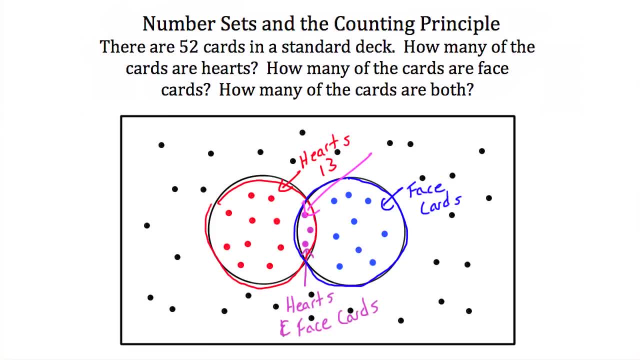 are both hearts and face cards. But what if we wanted to know how many cards are hearts or face cards? Well then we could count the dots. We could do 13 hearts, We could do 13 plus 12. That would get us 25.. But that's not actually the amount of 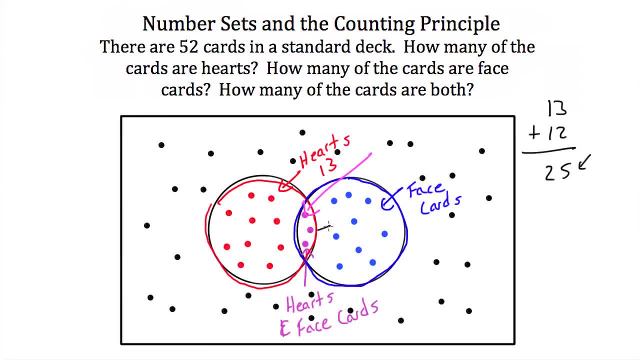 cards that are either heart or face card, Because what we've done is count these three points in the center here twice. We counted them when we counted our 13 hearts, and then we counted them again when we counted our 12 face cards. So we have to subtract 3 from 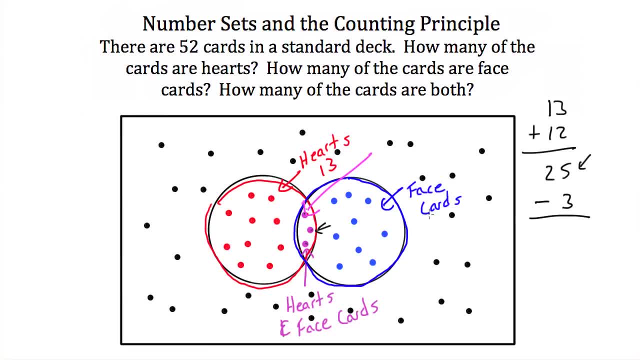 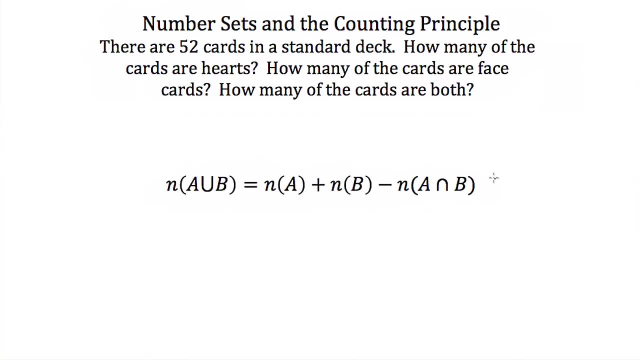 this total. But what we have to do, we gotta take off the 3 that we counted twice. So really there are 22 different cards that are either a heart or a face card. Now there's another way to illustrate this addition and subtraction that we just did. 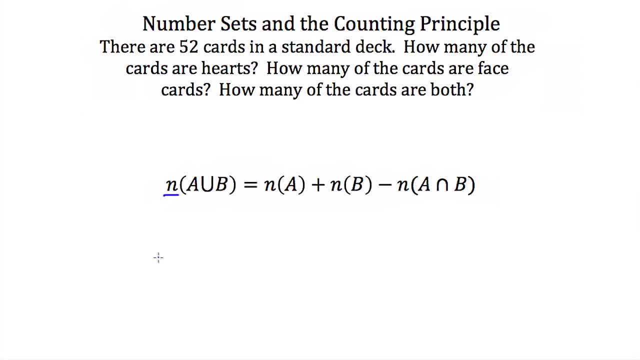 This first term here. this is the number, And then this a, with this crazy U and a- B. this means the union of A and B. This means anything that is A or B, Or you can think of a heart or a face card. So this would be the number of. 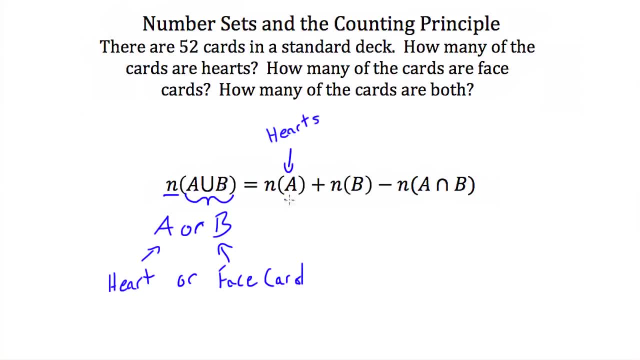 hearts. This would be the number of face cards, And then this number of A, and this is called the intersection of B, But you can think of this as A and B if you want. This is the number of cards. that would be hearts and face cards. 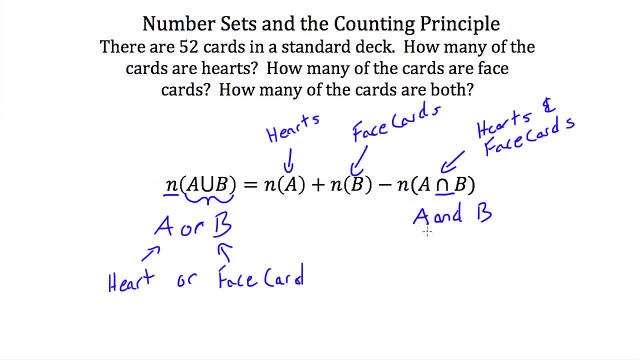 at the same time. So if we wanted to know the number of cards that are a heart or a face card, well then we would add up the number of hearts, which is 13,, and we would add that to the number of face cards- Well, there's 12 of those- And then we would subtract the number of cards. 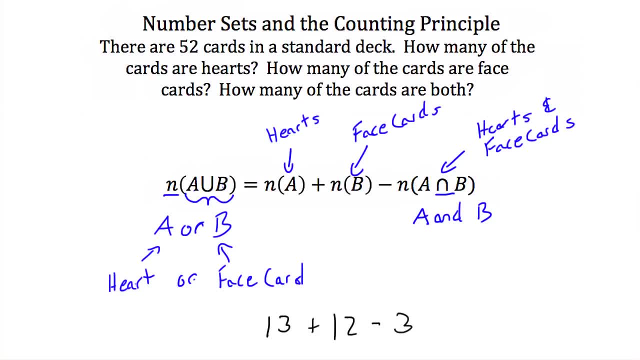 that are both hearts and face cards. Well, there are three of those. This brings us back to our 22. So the number A would be 22, or the number of hearts or face cards would be 22.. This is a popular way to 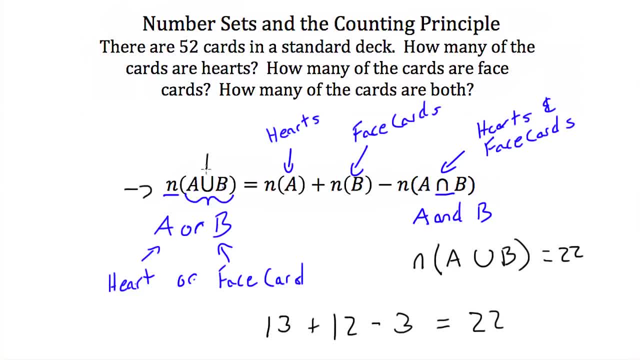 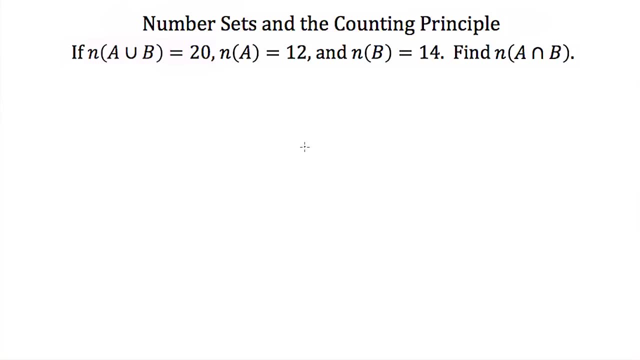 write our formula So recognize what this union and this intersection and the difference of what these two things mean. One is or and one is. and Now, frequently we'll be given different elements of this formula and asked to solve for them when we bring same- seus both to the same equation or the same. 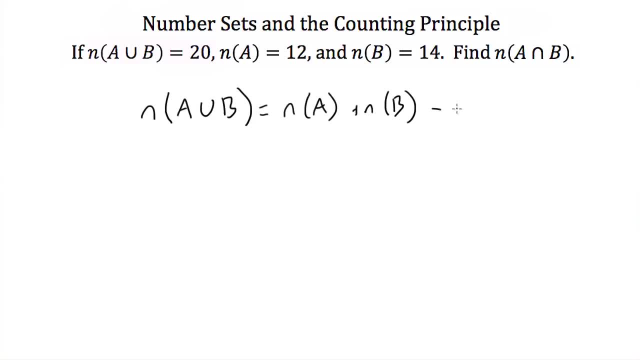 equation before And remember this section: given their numbers means the number they're从 A to B, And we wanna find the number is 20.. This should equal to the number A, which we're also given, and the number B we're also given, And we want to find the number after A and B And we want to find the number between A and B and we…. 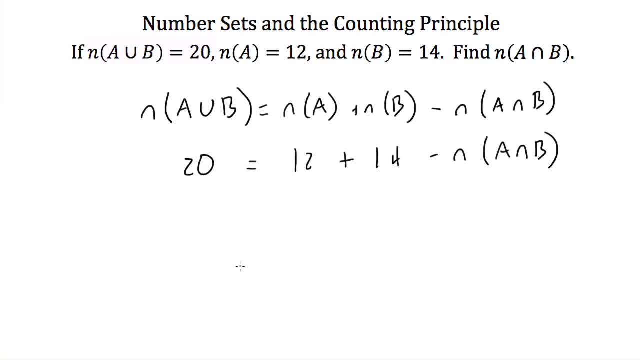 intersection B. Well, we have 20, and that's equal to 12 plus 14, so that's 26, and then we're going to subtract the intersection of A and B. If we rearrange this, we'll find that the number of elements in the intersection of these 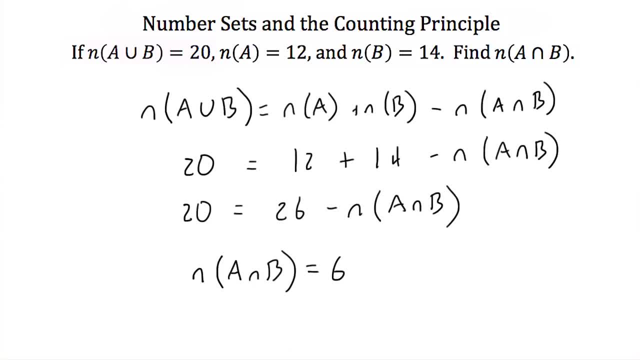 two sets A and B. well, that's equal to 6.. Now you may be given any different number or every different element of this equation, but usually it's just an addition and you just have to solve for the missing part. In this case, we solve. 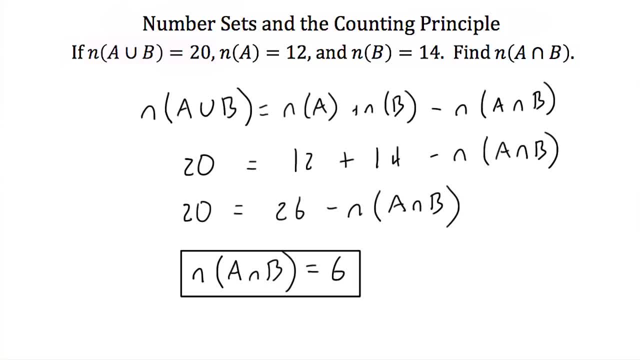 for the intersection, and that was equal to 6.. Sometimes we'll be given a Venn diagram illustrating the difference between the two sets. If we're given a Venn diagram illustrating the difference between the two sets, If we're given a Venn diagram illustrating the 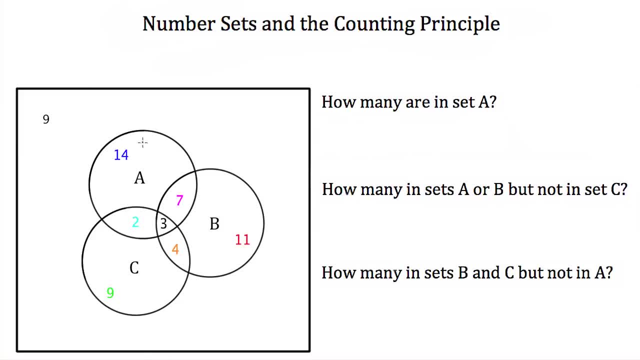 number of different elements in each different set. We have set A, B and C in this Venn diagram and these numbers illustrate the amount of elements in each set. So there are nine elements, not in any of the three sets. There are 14. 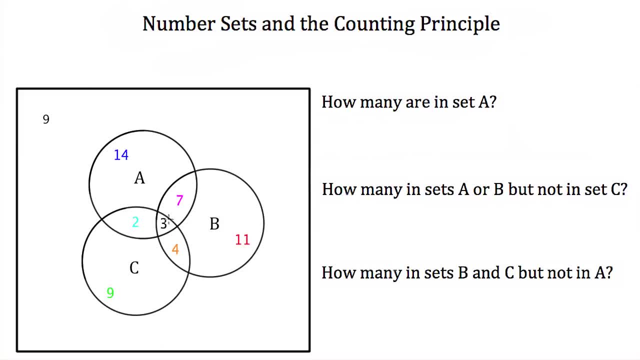 elements just in set A. There are three elements here that are in set A, B and C. So we're asked: how many are in set A? Well, there are the 14 that are in set A, but there are also seven that are in set A and B. Well, these are still in set A. so 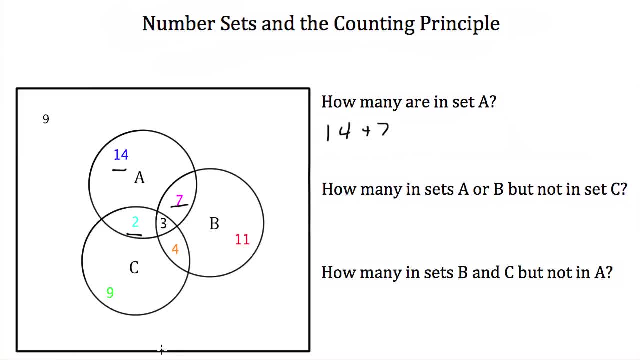 we'll add them to the other 14.. There's also these two here that are in both sets A and C, but they're still in set A, so we can add the two to there. And then we also have the three here that are in set A and C. 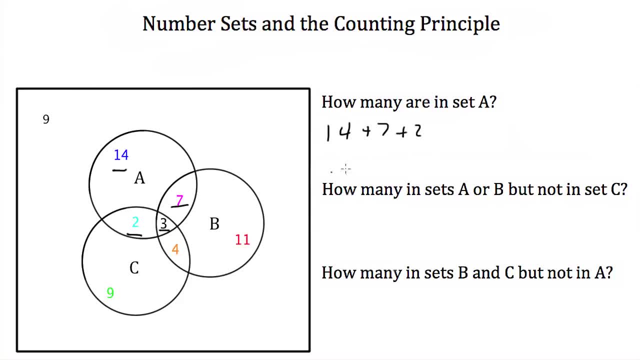 are in set A, B and C, So we can add the three to that, because those are also in set A. So 14 plus 7 plus 2 plus 3, that's 26.. So apparently there are 26 elements in set A. Now we want to know how many are in set A or B but not in set C. So 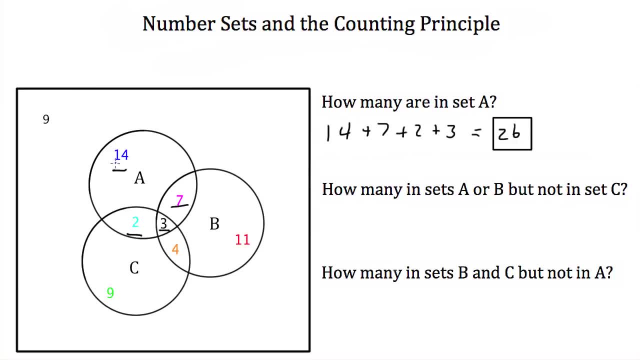 sets A or B. well, these 14 are in A, these 11 are in B. We have these seven here that are in A and B. We have these two that are in A and C, but our elements cannot be in C, So we 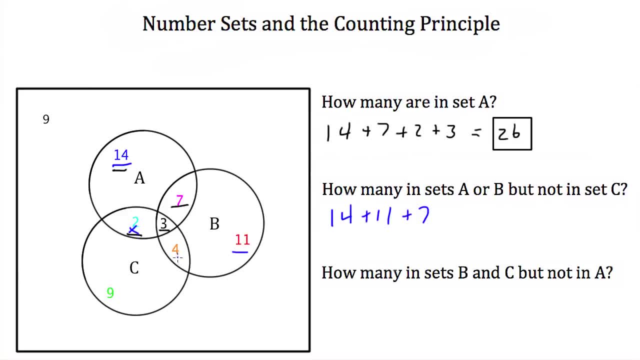 ignore those. We have the four here that are in B and C, but they can't be in C, so we ignore those. and then we have these three here that are in A, B and C, but since these are in C as well as in A and B, we cannot use those either. so how many? 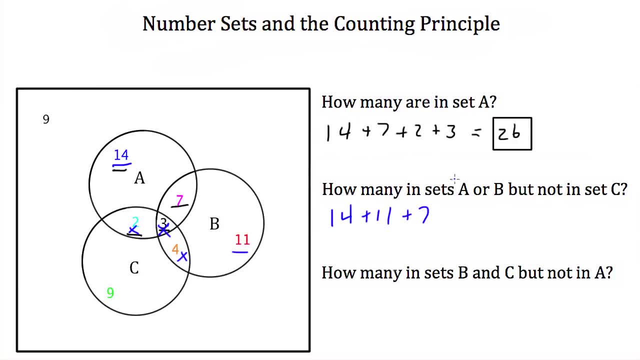 elements are in set A or B but not in set C. well, 14 plus 11 plus 7, so there are 32 different elements in set A or B, but not in set C. now, lastly, we're asked how many are in sets B and C but not in A? so for a set to be valid, it has to be: 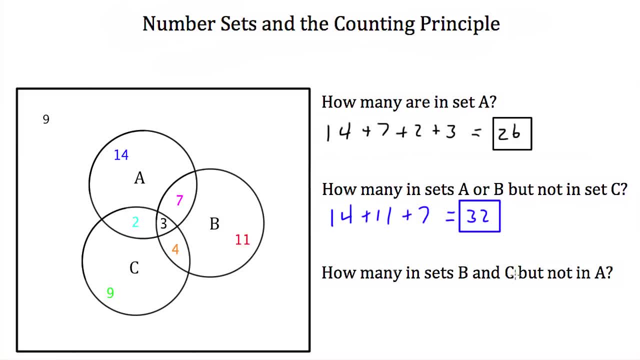 in both B and C, but not in A. so let's find all all set A and B and B, but not in A. so let's find all all set A and B and B and C, but not in A. so let's find all of the possible elements that are in both B and C. That would be all of these elements. 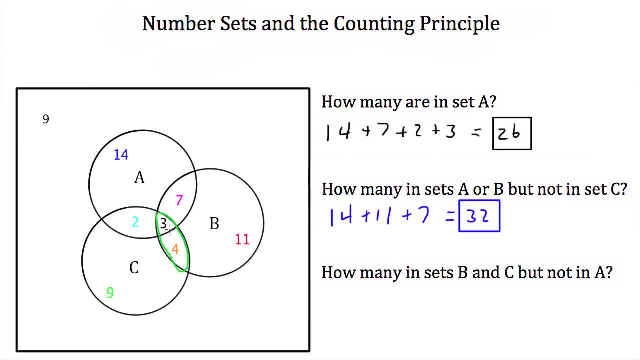 Three of these elements, though, are also in set A, and we've decided to exclude them, but not in A, So these don't count. So how many are in sets B and C? Well, four different elements are in both B and C, but not in A. So that's how you use a Venn diagram to determine how many elements are in. 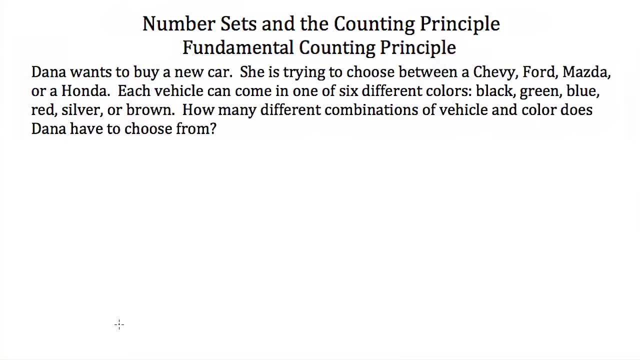 the different sets. Now the last thing we have to talk about is the fundamental counting principle. And let's look at this example situation Here. Dana wants to buy a new car. She's trying to choose between a Chevy, a Ford, a Mazda or a Honda. Each vehicle can come in one of six different. 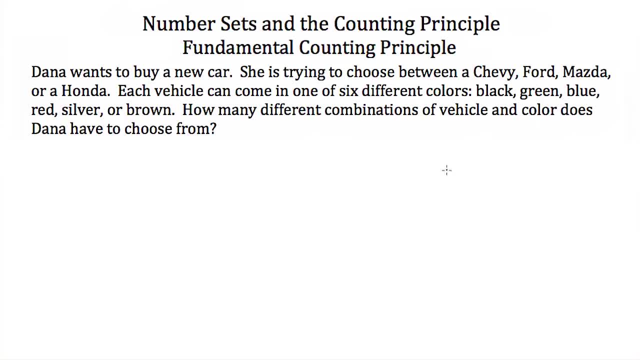 colors: Black, green, blue, red, silver or brown. So how many different combinations of vehicle and color does Dana have to choose from? Well, here's Dana, and she can choose between a Chevy Ford, Mazda or a Honda. So she has four. 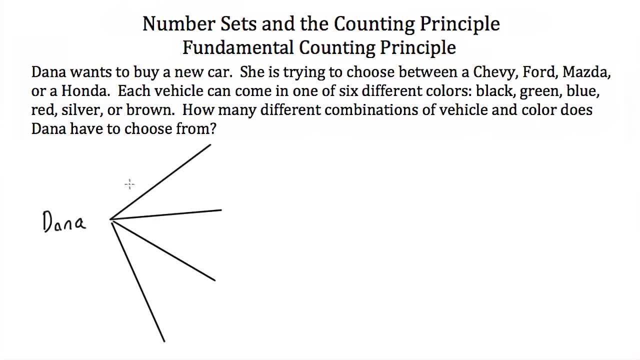 different choices. She can choose a Chevy, a Ford, a Mazda or a Honda. One choice is a Chevy, a Ford, a Mazda or a Honda. Once she's chosen between the four different makes of car, she has six different colors to choose from. 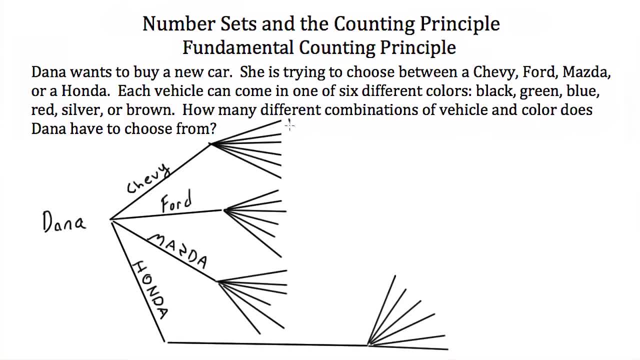 If she chooses the Chevy, she can get a black Chevy, she can get a green one, a blue one, a red one, a silver one or a brown one, And she has the same six choices. if she chooses the Ford- Black, green, blue, red, silver and brown- And if she chooses the Mazda, she can get a black one. 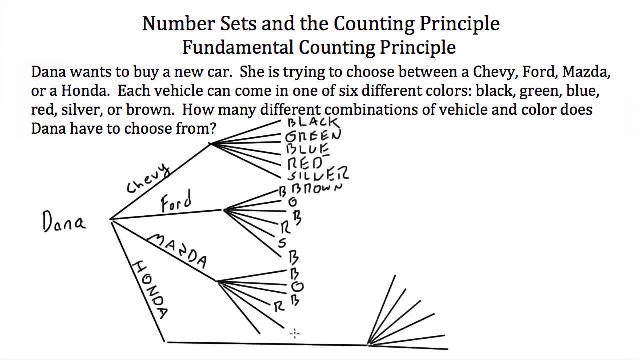 a green one, a blue one, a red one, a silver one or a brown one. And if she chooses the Honda, she can get a black one, a green one, a blue one, a red one, a silver one and a brown one. 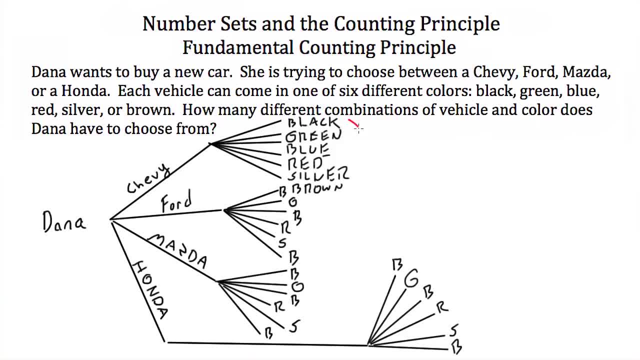 Now, if we count up all of these different options, there are six here, six there, six there and six here. So there are 24 different possible combinations of vehicle and color that Dana has to choose from. First she had to choose between four different makes of car, and then she had to choose. 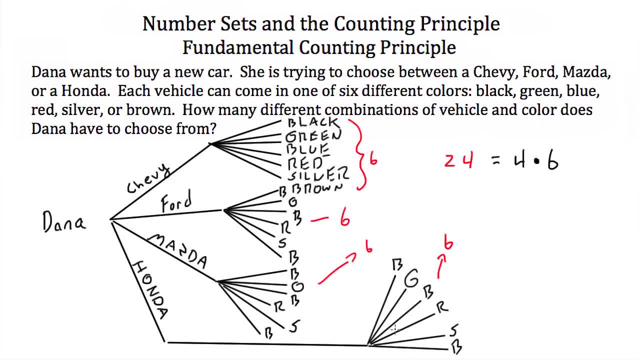 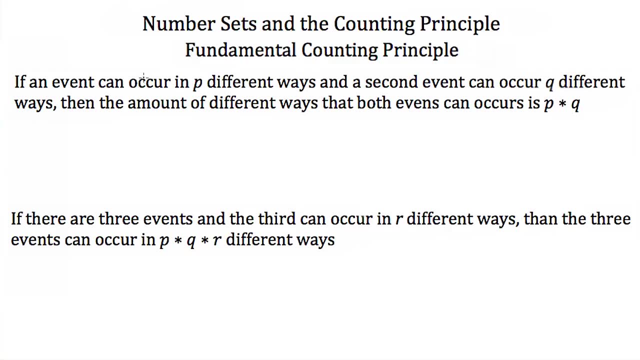 from six different colors of those cars. Multiply four and six and you get your 24.. This is the fundamental counting principle. The fundamental counting principle basically states if an event can occur in p different ways, the event would be Dana choosing the type of car. 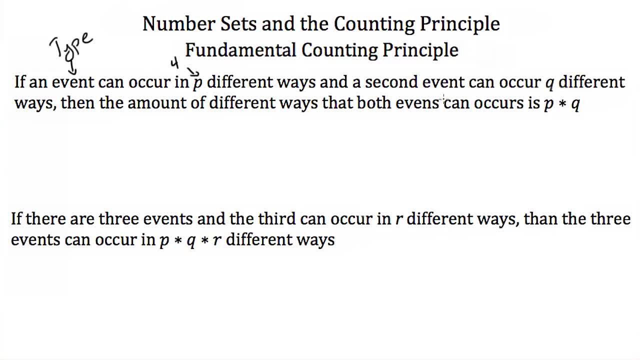 which occurred in four different ways, And a second event can occur in q different ways. You can think of this second event as choosing the color, And that can occur in q different ways. Well, there were six different colors to choose from, Then the amount of different ways that both events can occur is p times q. 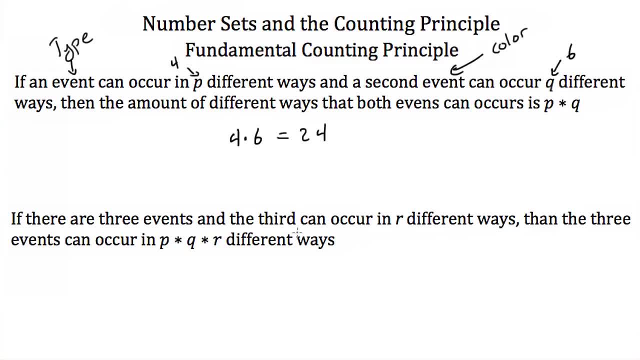 Four times six is 24.. Now if there are more than two events going on, then you just keep multiplying And you start multiplying the different ways that each one can occur. So if there are three events and the third one can occur in r different ways. 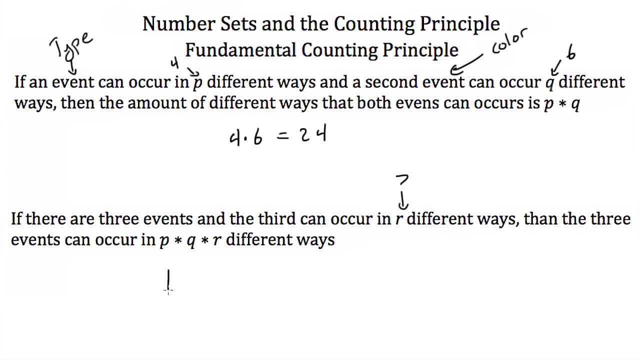 say r was seven, then the three events can occur in four times, six times seven different ways, And that would be 168 different ways of choosing between the three possible events or the three possible choices. So let's look at how we can do that. 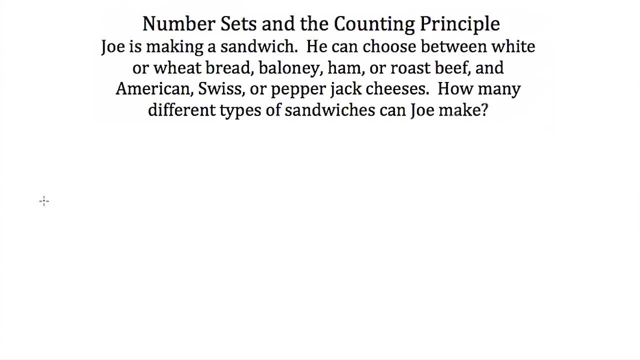 at an example Here. Joe is making a sandwich. He can choose between white or wheat bread, bologna, ham or roast beef, and American, Swiss or pepper jack cheeses. How many different types of sandwiches can Joe make? Well, we have Joe and he's going to make a sandwich, His first choice. 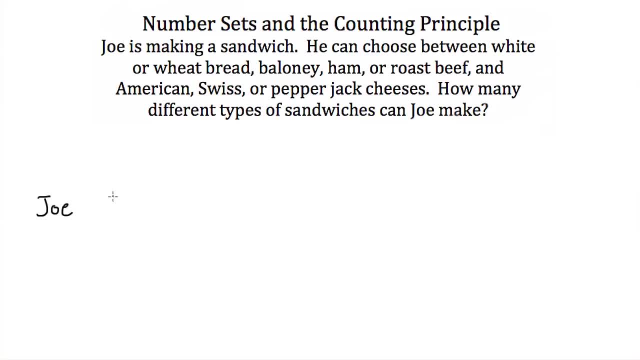 is to choose between white or wheat bread. So there are two different choices on the bread. There are three different choices of meat: bologna, ham or roast beef. So after we choose what type of bread, we have three different choices between the bologna ham or roast beef. 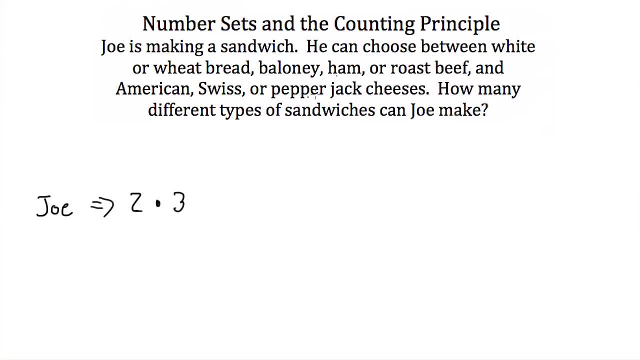 And then, lastly, we have three different choices of cheese to put on the sandwich: American, Swiss or pepper jack. So since we have three different choices, we multiply this by three. So how many different types of sandwiches Can Joe make? Well, he can make two times, three times, three different types.